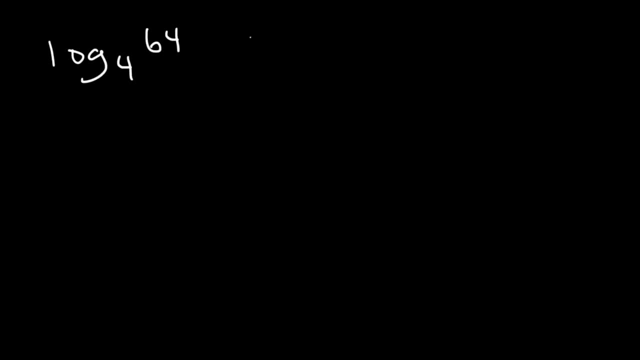 Convert the following logarithmic expression into its exponential form, And you can try this one as well: 4 raised to the third power is equal to 64. So that's how you can write it in exponential form: 8 raised to the second power is equal to 64. And so we can write it like this: 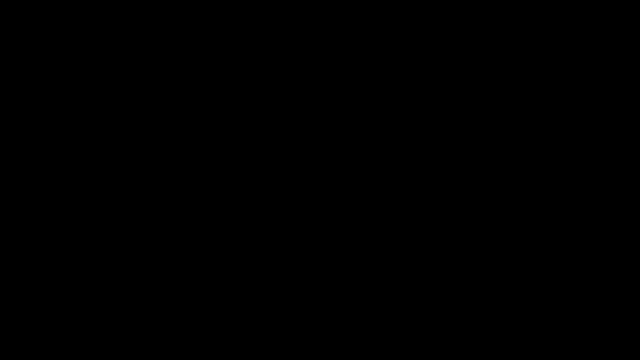 Now what about the reverse? Let's say, if we have an equation in exponential form, Convert it to logarithmic form. Try these three examples. Feel free to pause the video. So the base is 2.. The base is the one with the exponent. 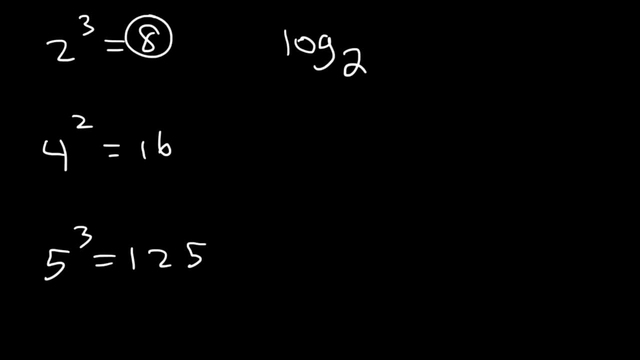 So log base 2.. And what is across the equal sign? We'll go here. And the logarithmic function always equals the exponent. So to check it, you can see that 2 raised to the third power is equal to 8.. 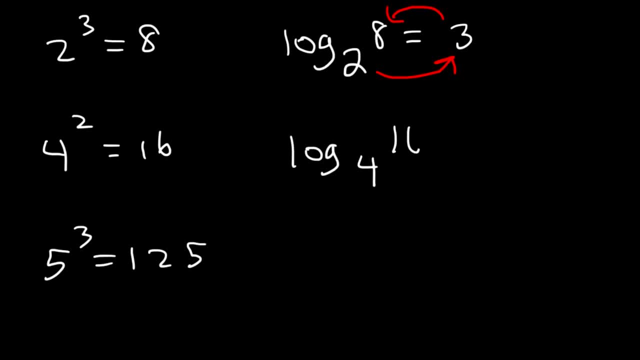 The next one is going to be log base 4 of 16 is equal to the exponent which is 2.. 4 raised to the second power For the last one, log base 5.. The base is the one with the exponent of 125 is equal to the exponent of 3.. 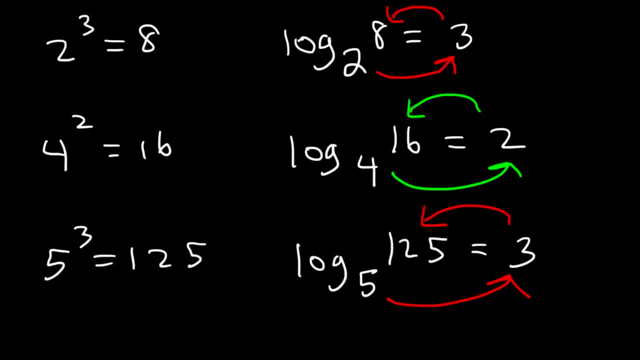 5 to the third, power is equal to 125.. The next one is going to be log base 5.. The base is the one with the exponent of 125..